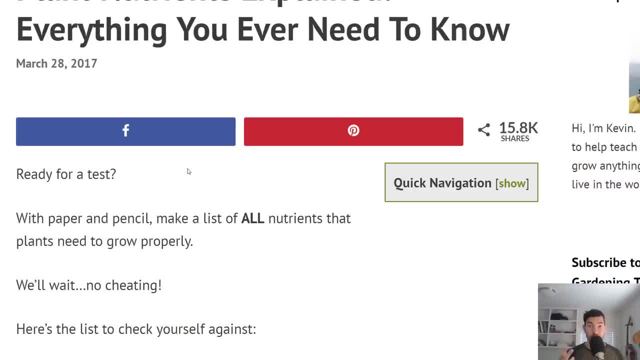 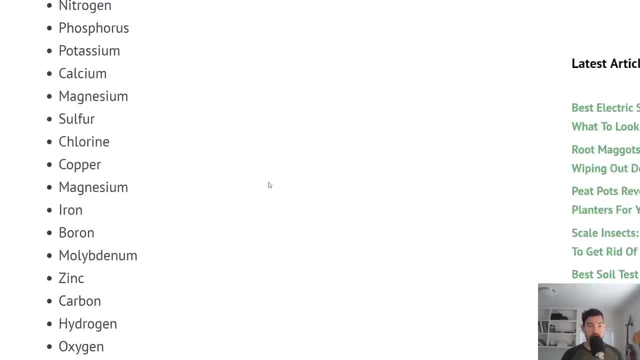 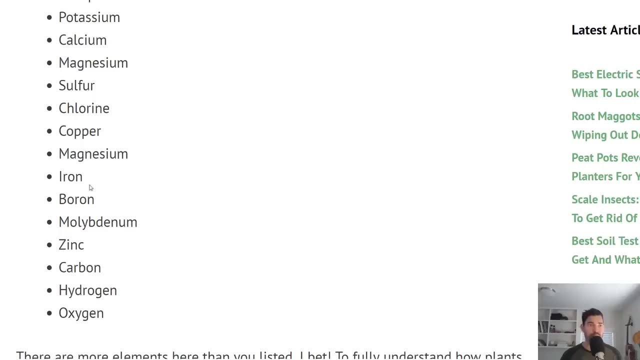 make a list of all the nutrients you think a plant needs to grow properly, thrive and survive. So write it down. and then here's the real list to check yourself against: Boom Nitrogen, phosphorus, potassium, calcium, magnesium, sulfur, chlorine, copper, magnesium, Oops. 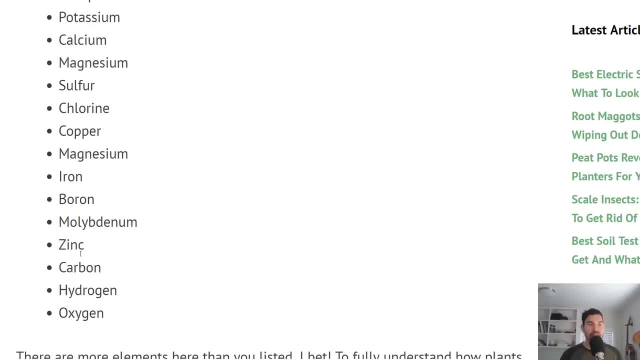 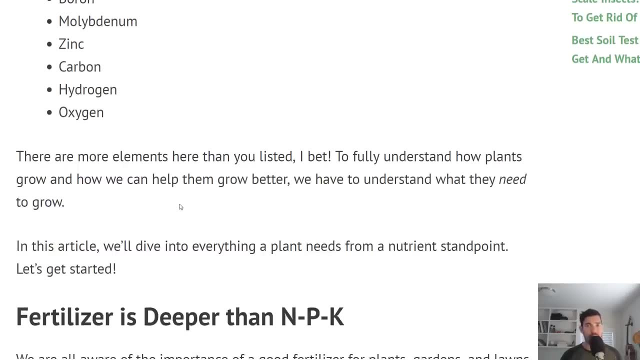 I have that Twice: Iron, boron, molybdenum, zinc, carbon hydrogen oxygen. There's a lot of stuff. Those are all elements right, More than you would probably have listed, unless you are a botanist. 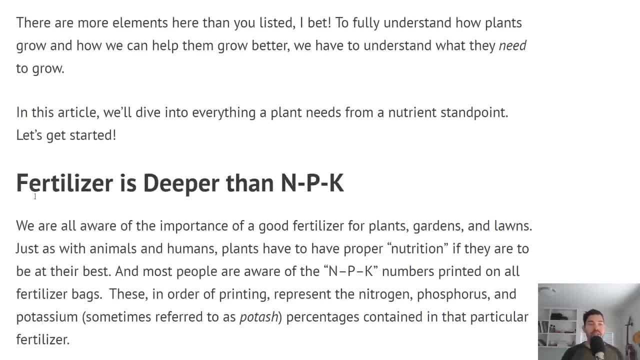 right. So here's what we need to understand. Fertilizer is much deeper than NPK. Those are the numbers we see on a fertilizer container. It is much deeper and more complex than that And we don't need to know every intricacy to get a good understanding of how to grow plants. but 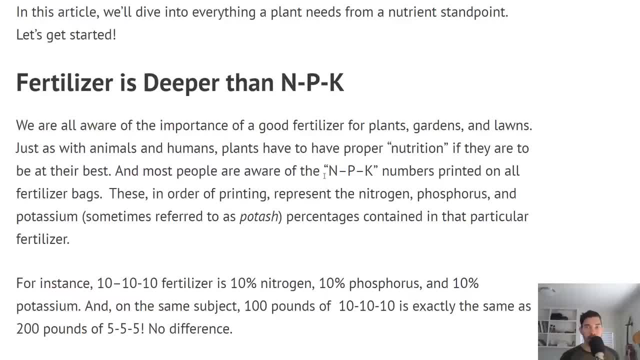 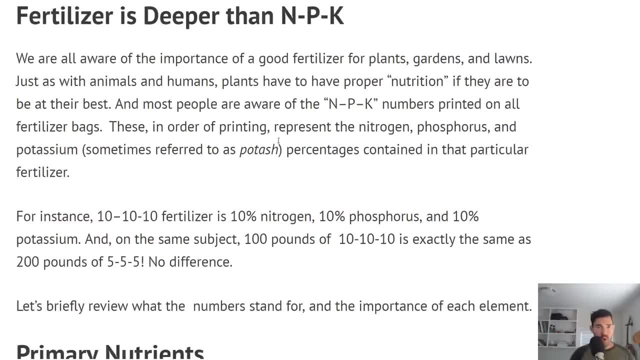 we do need to get a base level so we can say, hey, what's going on with my plant? Maybe it needs more of this, Maybe it's not having has enough of this. Let's keep talking. So we are all aware. 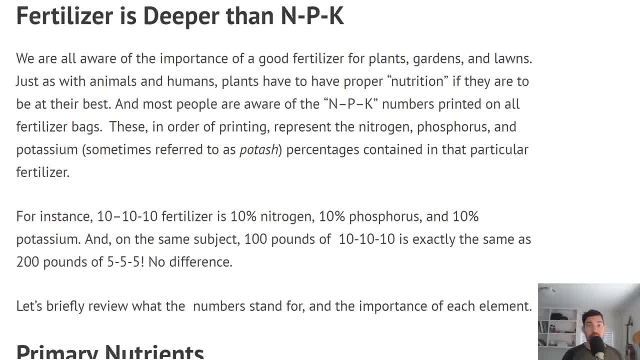 that plants need a good fertilizer, and whether that's coming from organic matter in your soil as you build it over time. whether you're buying organic nutrients, whether you're doing synthetic nutrients, plants need it. That's just a fact of life, right? So let's talk about the NPK numbers. 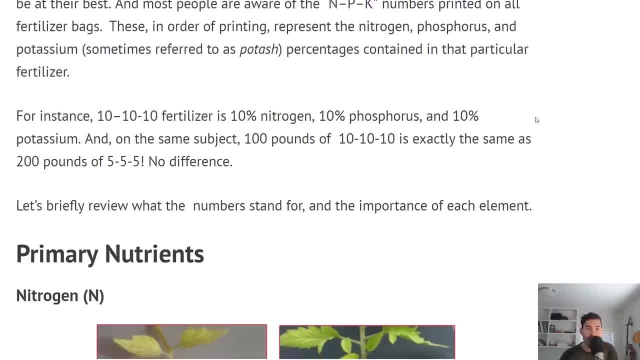 A 10, 10, 10.. That's 10% nitrogen, 10% phosphorus and 10% potassium, right? And so 100 pounds of 10, 10, 10 is the exactly the same as 200 pounds of 555, because it's a percentile, right, And so you're going to get 10 of each of. 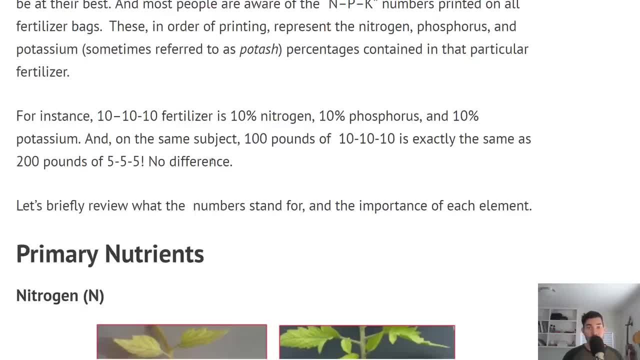 these and you're going to get 5% of 200, which is also 10 of each of these, right? So there's no real difference there. That's one thing that I think can trick people, And so let's talk about. 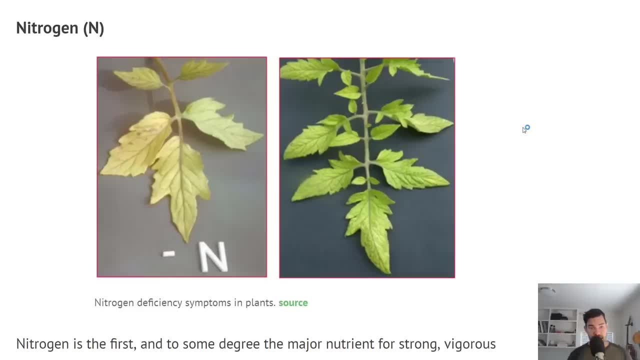 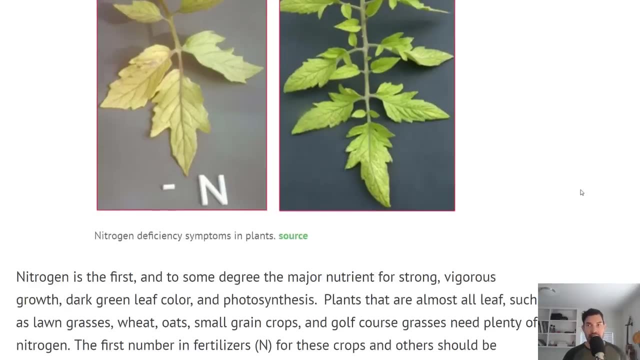 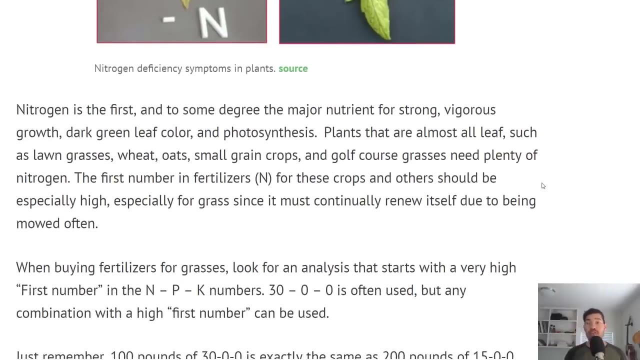 the primary nutrients. first, Nitrogen, the granddaddy right. This is a symptom, This is a just, so you can see. you get a lightness, a light greenness to the plant And so this is one of the most important nutrients for strong, vigorous growth. dark green leaves a lot of the processes. 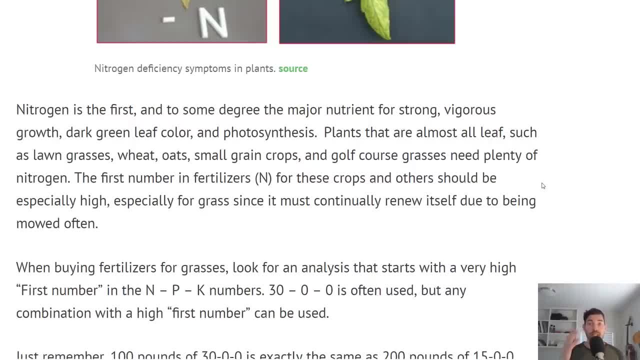 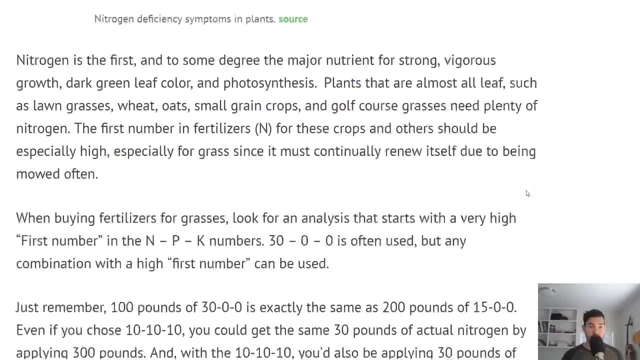 within photosynthesis. So plants that we're going to grow for mostly their leaves, their vegetation, grass, wheat, oats, leafy greens, microgreens, et cetera- they need a lot of nitrogen, And so when you're buying a nitrogen based fertilizer for plants, you're going to want a high first number. 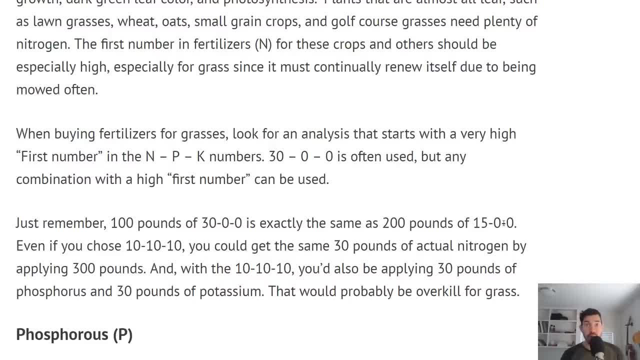 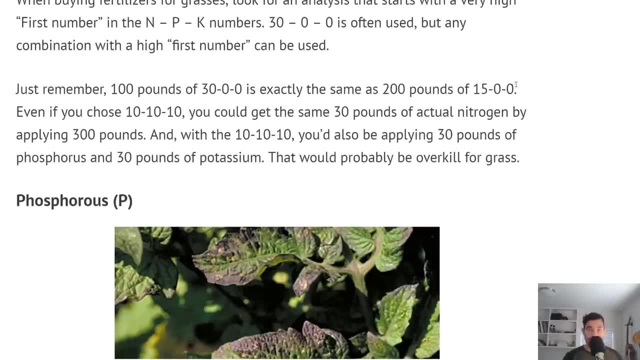 30, 0, 0 is what people will use for grass, Because, again, grass is pretty much all vegetation, right, It's all leaves. Just remember that rule. a hundred pounds of 30, 0, 0 is the same as 200. 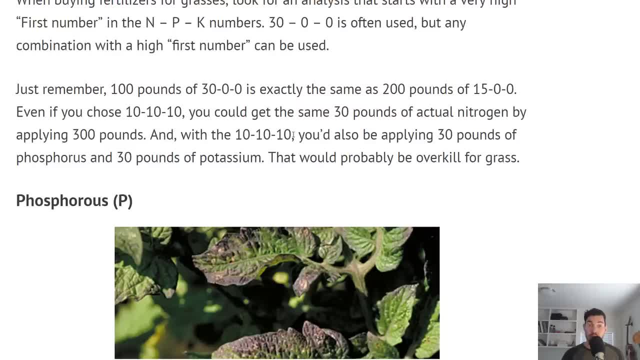 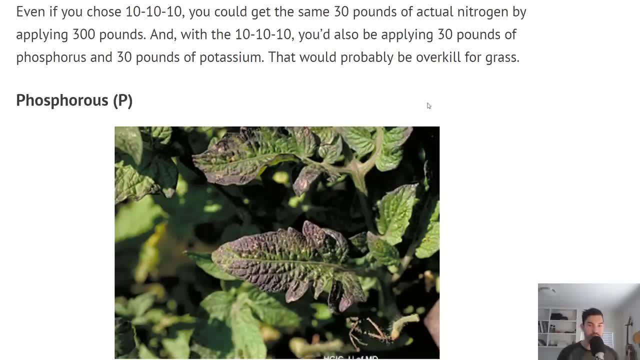 to 15, 0, 0.. And so you know, work, work on that, work on those math skills there If you want to make sure that you have a good grasp on what you're actually buying when you buy these fertilizers. 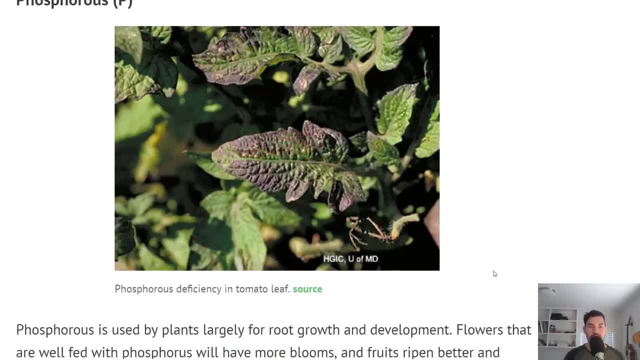 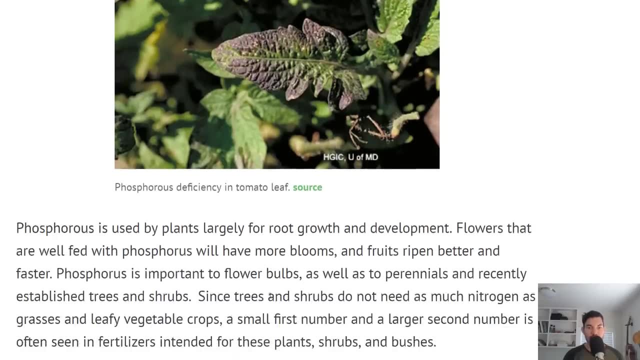 All right, let's talk about phosphorus now. So here is an example of phosphorus deficiency in a tomato leaf. You can see it has that sort of purplish reddish coloration there. Phosphorus is really used for root growth and development. 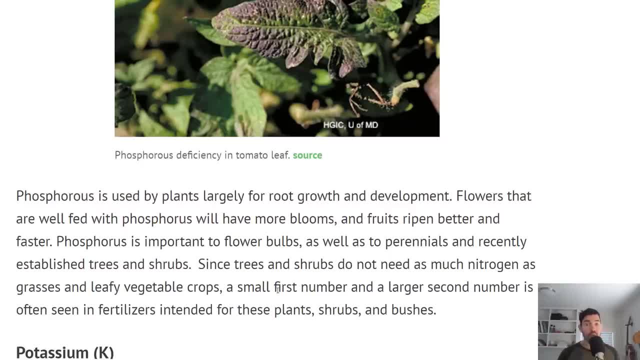 So flowers that are fed with phosphorus will have more blooms. fruits ripen better and faster. It's very important to flower bulbs, as well as to perennials and trees and shrubs- So effectively all plants- but it's important to know specifically what a plant will use it for. 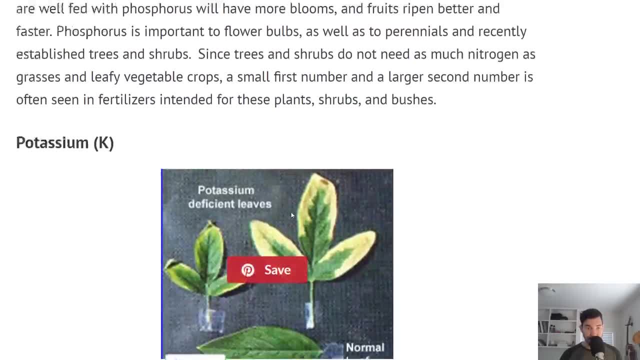 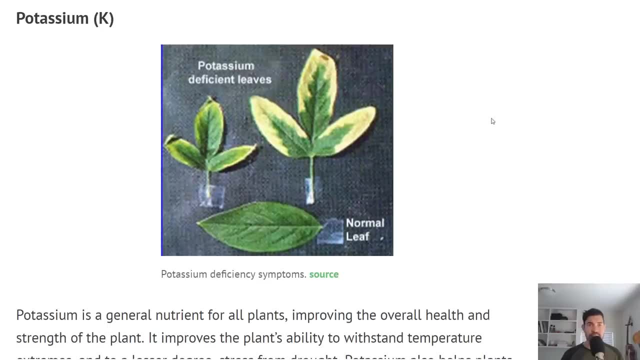 so we can see what's going wrong. right, All right, potassium. Here is an example of a normal plant. So it's a plant that has been growing for a long time. It's got potassium deficient leaves, So you can see this yellowing start to creep in from the outside of the leaf towards the interior. 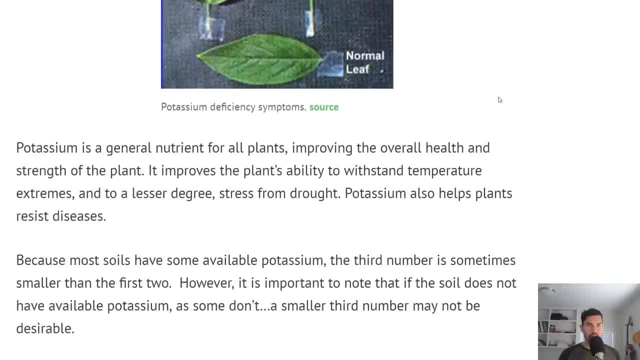 And that's a very clear symptom of potassium deficiency. So potassium it's a general nutrient for all plants, being one of the big three improving overall health strength the plant. It's a temperature regular, it helps the plant withstand temperature extremes and it also helps 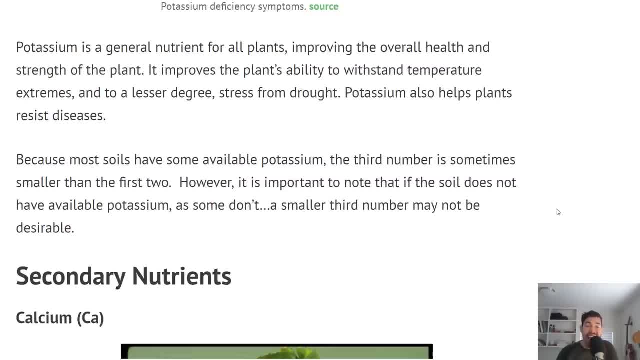 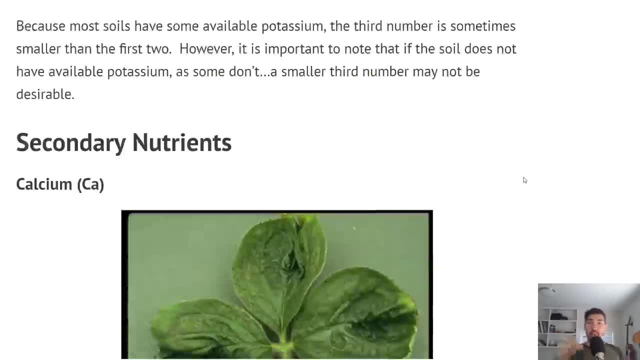 resist diseases. So, a lot of the times, Most soils are going to have a good amount of potassium in them, And so the third number is sometimes a little bit smaller than the first two, but it's important- if you looked at my video on soil tests- to test your soil. 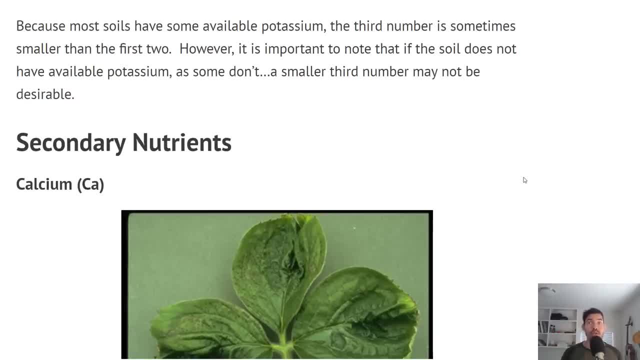 you're going to. you need to know what's in your base level soil So you know what your plants are going to be short in or maybe have a surplus of, because for all deficiencies there are also toxicities. You can have too much of a nutrient as well. 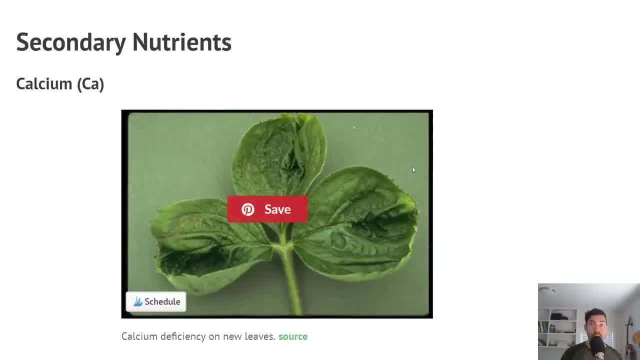 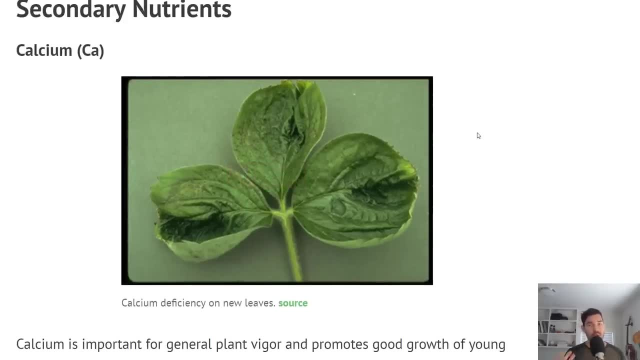 Very similar to us as human beings. You can have too little of a vitamin. You can have too much of a vitamin, right? Okay, Now we're getting into the secondary nutrients. These are the ones that most people don't have a good understanding of and don't. 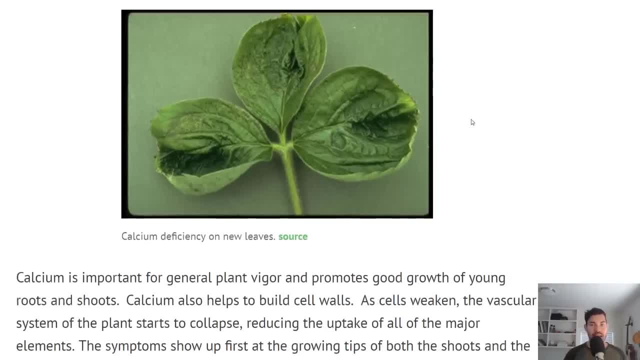 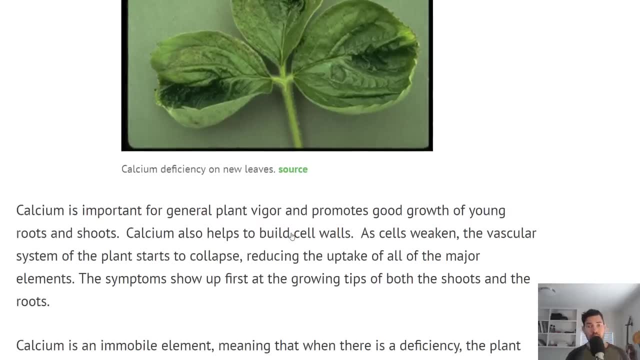 really understand how they impact the plant, And so here we're talking about calcium. Here's an example of calcium deficiency on some new leaves, So it's something that you can spot. It's important for plants in the in their younger stage of life. 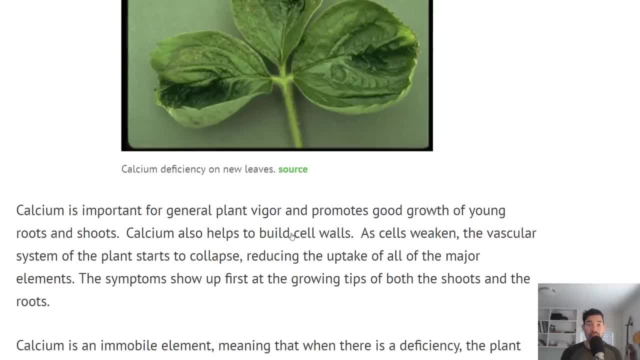 young roots, young shoots, helps build cell walls If you have a calcium deficiency. what you're going to see is the growing tips Those edges are going to are going to start to decay and collapse right. Calcium: it's an immobile element. This is what's interesting. 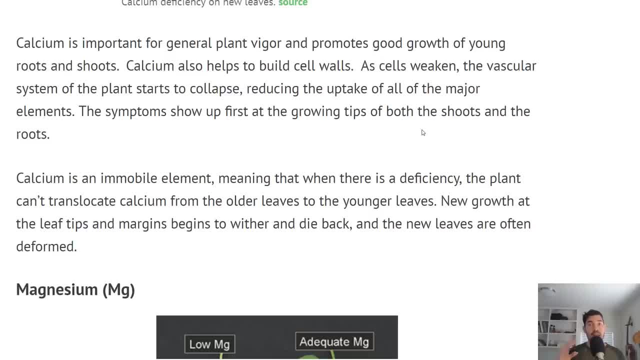 So when there's a deficiency in calcium, the plant cannot move calcium throughout its structures to get to these younger leaves that don't have it, And so calcium stays where it is in the plant, which means that a deficiency is going to show up on new growth. 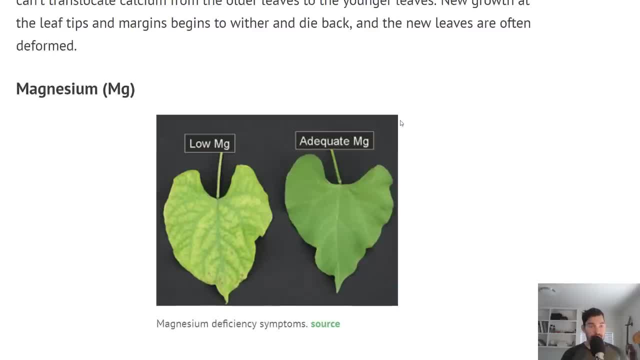 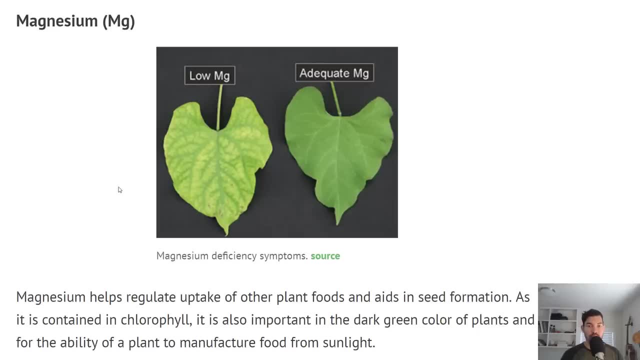 not old growth, right, That is a key for calcium deficiency. Okay, Now we're going to talk about magnesium, Magnesium. You can see here the deficiency symptoms. There is this sort of a veininess that appears in the plant. 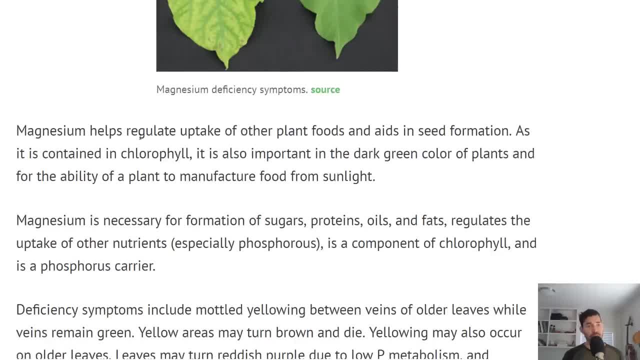 It's a little bit lighter in color And, as far as function, magnesium is going to help uptake other plant foods and aids in seed formation. Actually, it's actually something that's contained within chlorophyll helps plants get that dark green color in their vegetation. 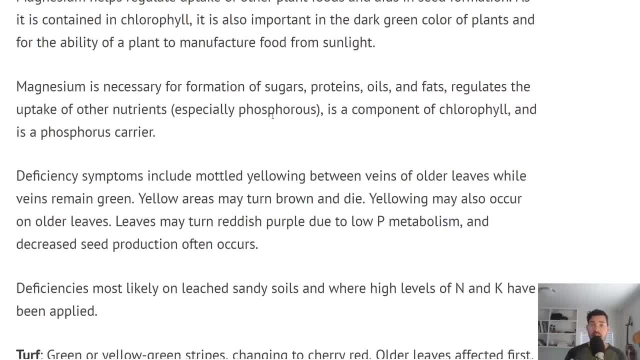 It is essential for a lot of the processes within a plant: creating sugars, proteins, oils, fats. uptake regulates the uptake of phosphorus, And so magnesium regulates the uptake of phosphorus, which is one of those big three nutrients. right? So deficiency symptoms. 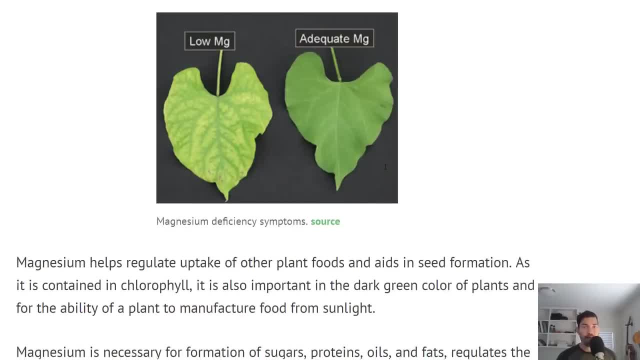 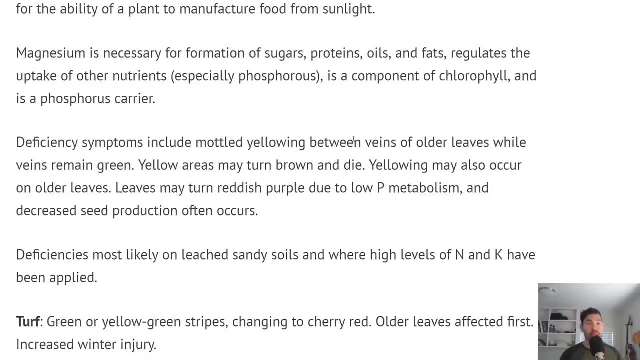 because this is what we're here for. How do we know what particular thing our plant is missing? Well, you know that by building a knowledge of what a plant looks like when it's missing a certain nutrient, So when plants are missing magnesium. 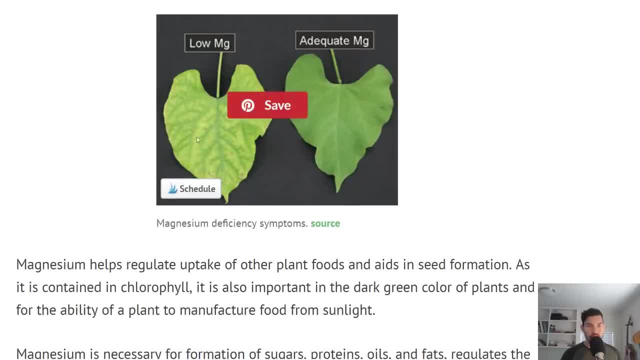 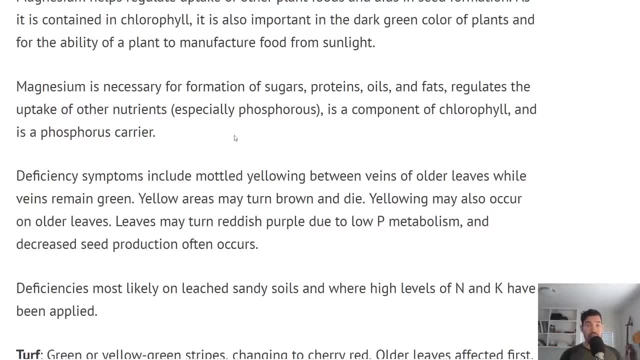 you have this mottled yellow. So look at this. You have this mottled yellow between the leaves, between the veins of the leaves, yellow areas. Eventually we'll turn brown and dye. They may actually even turn reddish purple because with low magnesium. 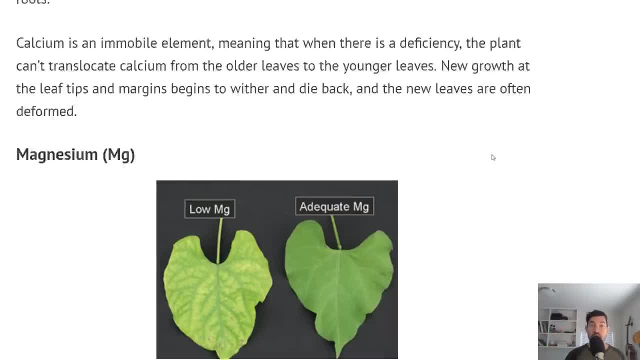 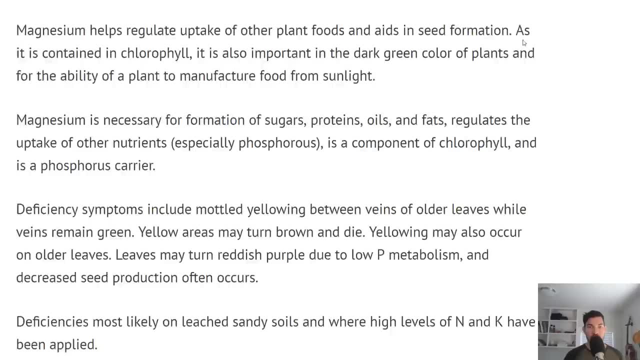 you're going to have poor uptake of phosphorus, right, And then you're going to get that phosphorus deficiency that we see right here, right, And so you can see there's a chain cause effect going on here. All right, There's some more stuff here about different, different deficiencies based on the. 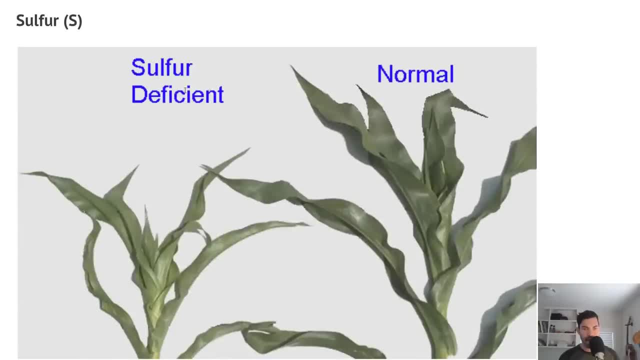 type of plant. but we'll get into that And if you want to look at it, of course you can just go to EpicGardeningcom Check that out. All right, we're going to get into soil Now. So here you can see a corn. sulfur deficiency in corn. 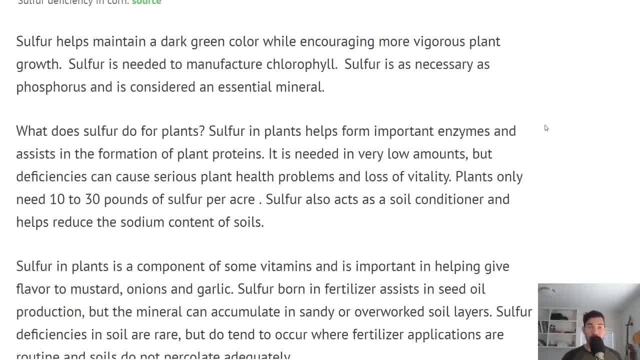 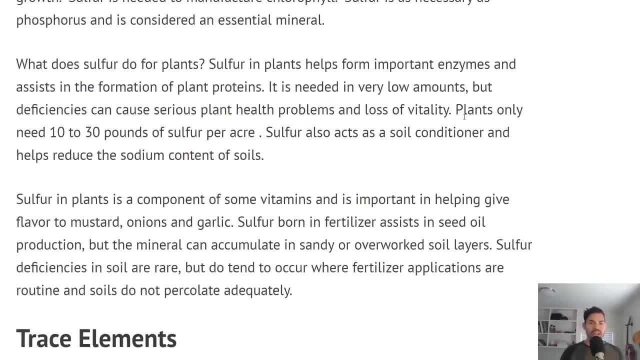 right And okay. What does sulfur do? again, Dark green color needs. it's needed to make. chlorophyll is as necessary as phosphorus and considered an essential mineral. Here's the thing, though: Like most, most soils have enough sulfur within them, and plants don't need a whole lot of. sulfur 10 to 30 pounds per acre, which is a very small amount. It's a soil conditioner. Honestly, very few people are going to run into a sulfur deficiency, especially if you're just growing at home. most of the soil is going to have it. 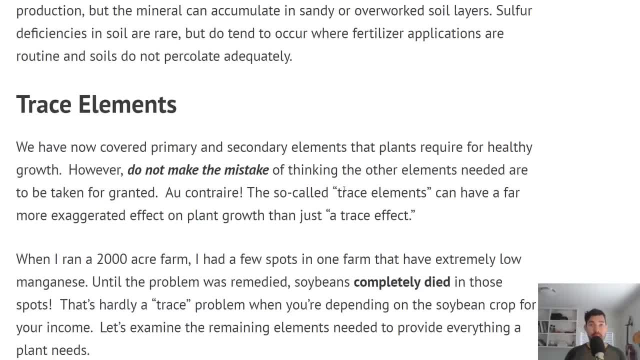 All right, let's move on to the trace elements. So we had our primary NPK, we had our secondary, which we covered just now, And now here are trace elements. So these are elements that plants need in very small effects, small amounts. 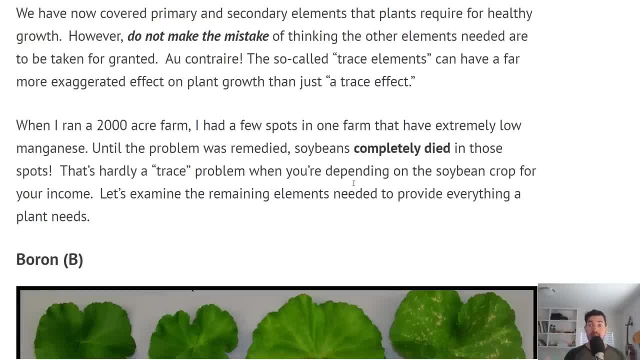 right. However, that does not mean that the absence of them is is not a big deal. The absence of a trace element can actually be quite drastic for your plants as well, right, Okay, So if you are depending on your crops to do well, 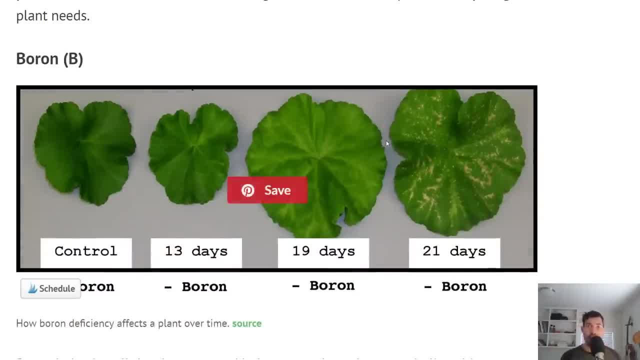 or you're just a gardener that wants your crops to do well. Yeah, If you're missing a trace element, you're going to have a hard time. right, You have a bad time. Okay, Let's talk about it, Boron. 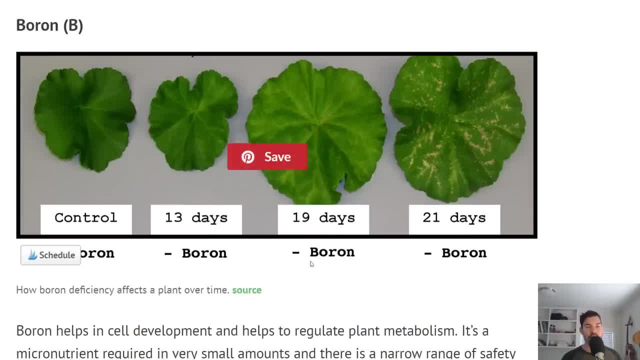 So here is an example of a controlled boron deficiency. This is an experiment, right? And so here's a a perfect plant. And then here's 13 days with boron deficiency, 19 and 20 days And 21.. 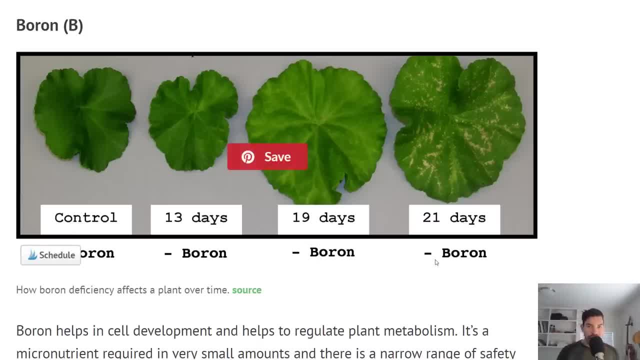 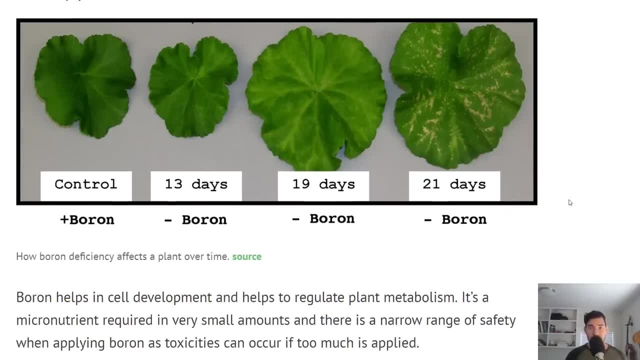 So what you, what you can see, is this yellow yellowing of the leaves. in between the veins You can see some spotting going on. It's actually quite a unique deficiency, So it's somewhat easy to identify. And what boron does is it helps synthesize protein. 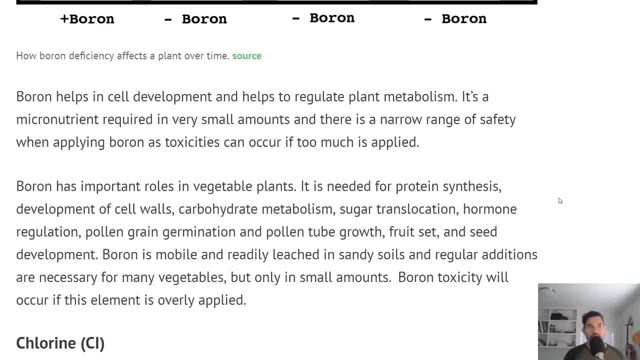 It helps develop cell walls. What you'll notice is a lot of these nutrients do a lot of things, as in they're used in conjunction with each other to to perform most of the processes for the plant. So that's boron. Let's talk about chlorine. 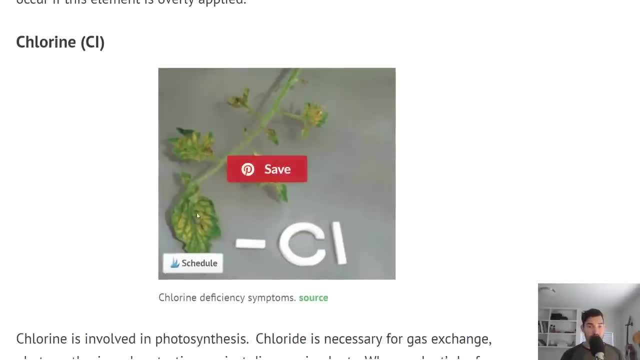 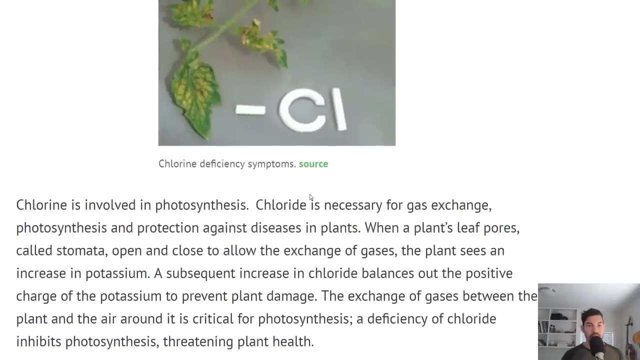 right. Chlorine is involved in photosynthesis. Here's a chlorine deficiency. It looks very similar to, let's say, a nitrogen deficiency. You're looking at a lightning and then some of this chlorosis in in the plant. Okay, Chloride necessary for gas exchange. 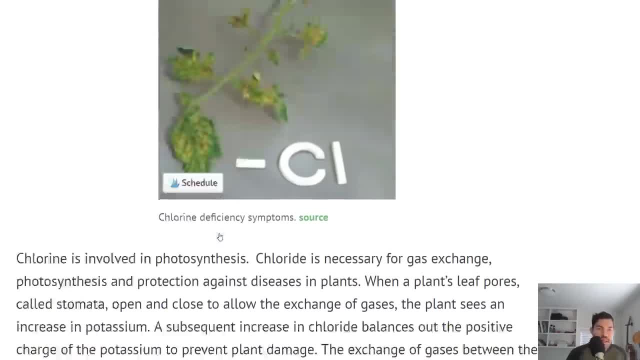 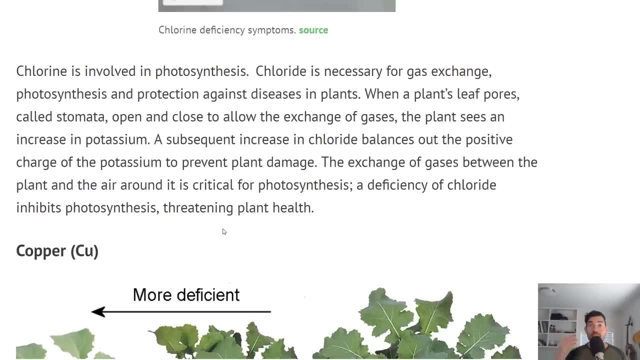 There. there's a whole lot I could go into about chlorine. Just just know that it's necessary and know for the most part you're not going to run out of this in your soil. Again, it's a trace element, which means a deficiency. 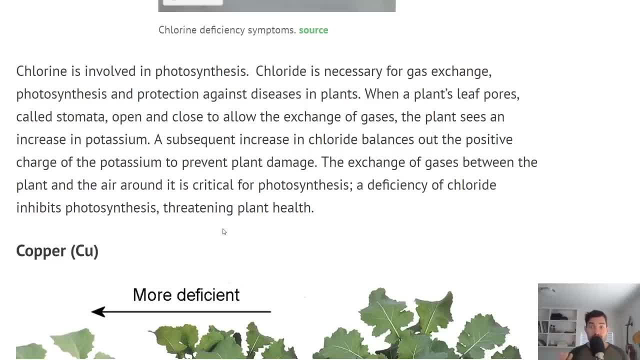 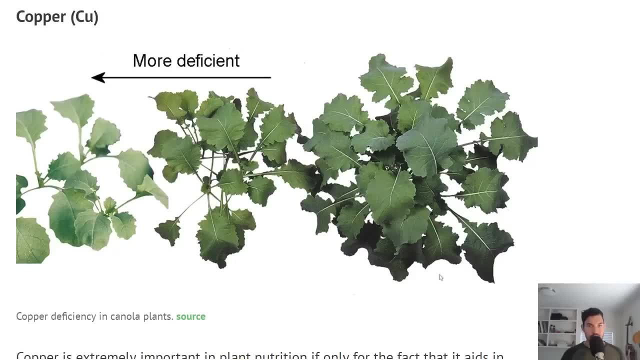 if you had of. it is rare, Although that deficiency is important If, if, if you don't have it right, Okay, here we go. Copper- copper deficiency. Here's an example of a copper deficiency in a canola plant. 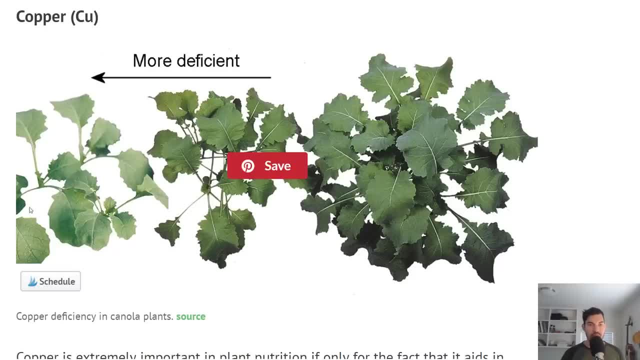 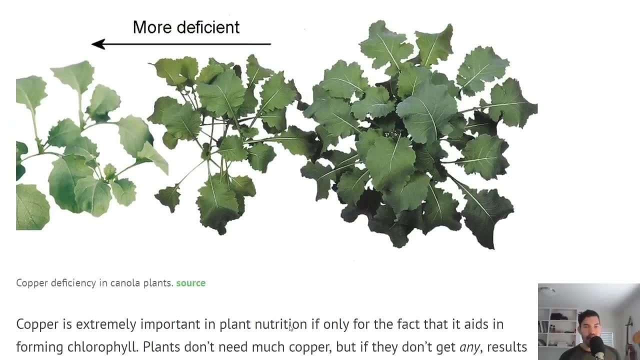 The image on the right being the most healthy. And then, as we move to the left, you get more deficient in copper, And so you're seeing a lightening of the leaf, and that is your symptom to look out for, Okay, Copper. 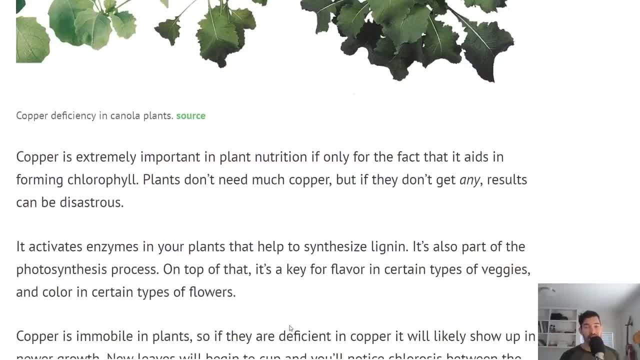 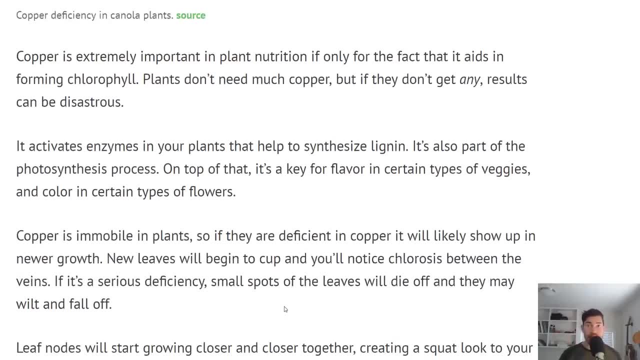 very important in forming chlorophyll. Plants don't need a lot of it If, again, it's a trace element. but if they don't get any, you got disastrous results right. Same principle across the board with all these plant nutrients. 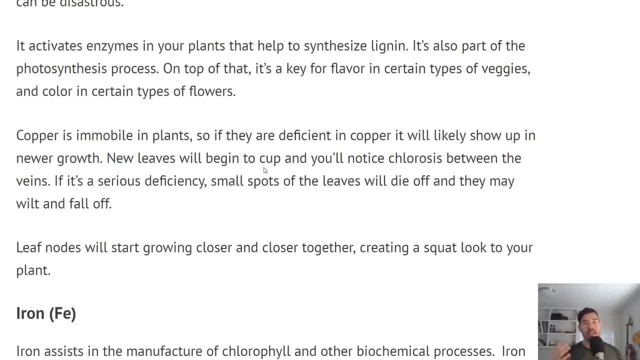 What it does is it activates enzymes in your plants. It helps to synthesize lignin. It's part of photosynthesis And, interestingly enough, it's key for flavor in certain types of vegetables and it's key for color in certain types of flowers. 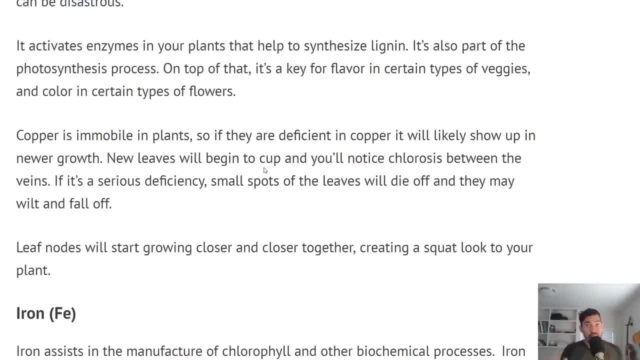 So, from a taste and aesthetic standpoint, even then you want copper in your plants. So again, copper is immobile. It's very similar to calcium, right? So if your plants are deficient in copper, it's going to show up in the newer growth, because plants cannot mobilize the 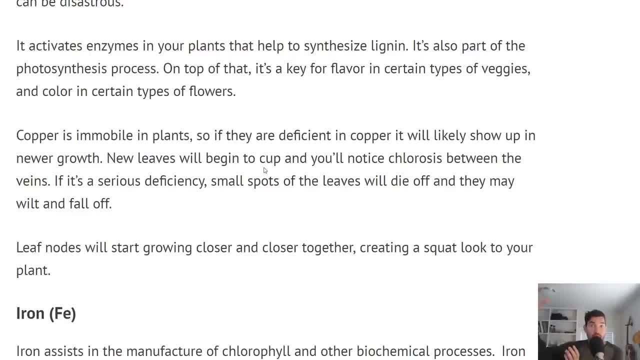 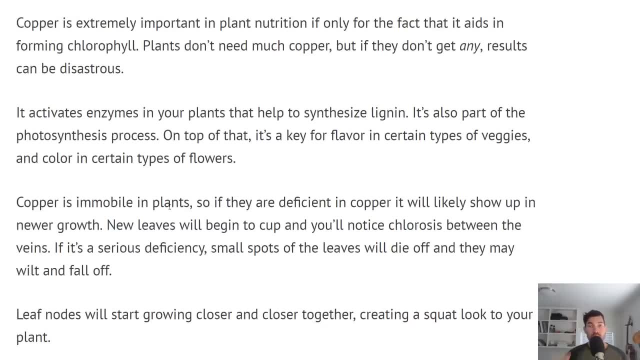 copper that is readily available in old growth to that new growth, like they could with other nutrients. Okay, Leaf nodes. This is an interesting deficiency symptom, leaf nodes. So the distance between new leaf growth on your plant, on the stem of your plan, is going to be shorter. 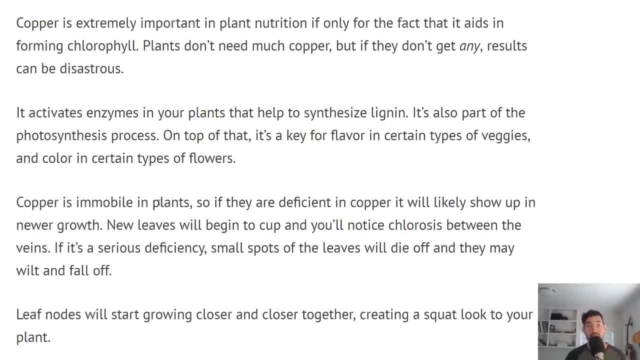 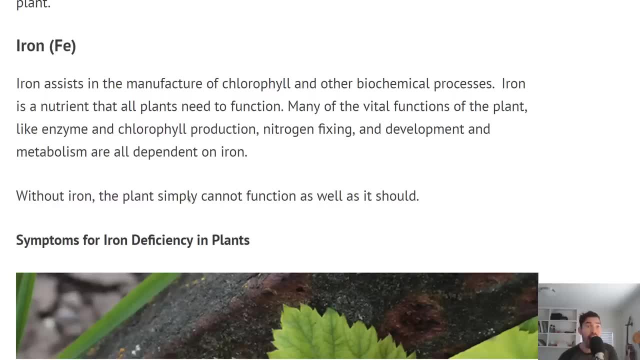 And so it's. you're going to get a more stout plant, uh, which is a interesting deficiency to look for. So there we go with copper. Now let's talk about iron. Iron assists in the manufacturer of chlorophyll, many other biochemical processes. 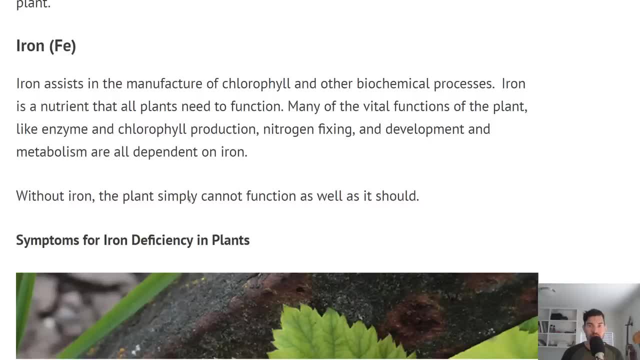 many of the vital functions of a plant- enzyme, chlorophyll production, nitrogen fixing and development of metabolism- all dependent on iron. So not a whole lot of interesting things to say here. Again, I'm not a botanist. This is just the information that I know I want to share and would be happy to have any comments. 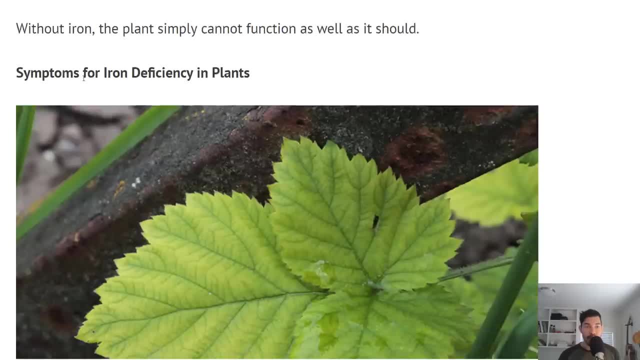 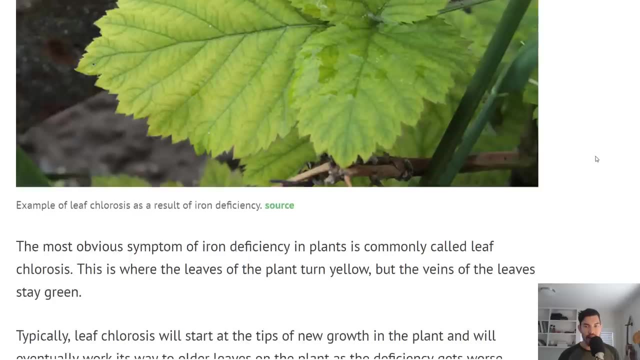 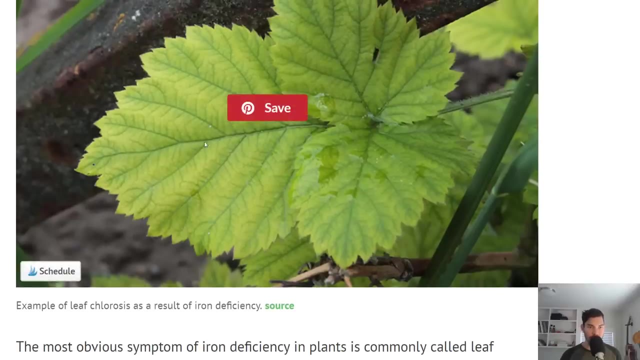 Um, there we go with iron, another trace element. here we can see a deficiency symptom, So leaf chlorosis, not a healthy looking leaf right there. So there you go. Leaves of the plants turn yellow, the veins stay green. So you can see if we trace along, these veins are green and the veins are much more apparent. 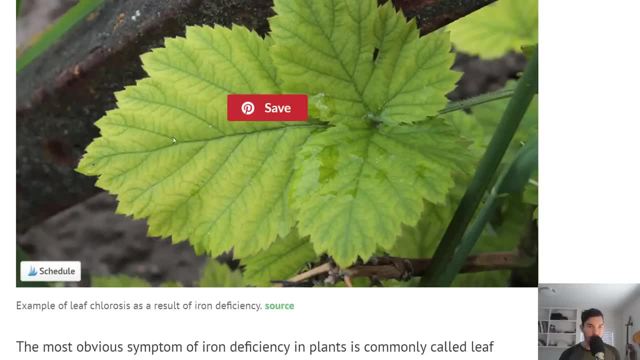 right, So you can see the main veins. Then you can see all these sub veins here, because the leaf structure has become so yellow, So the yellower is. imagine if your hand became translucent, you'd all of a sudden be able to see all these veins that you normally wouldn't be able to see. 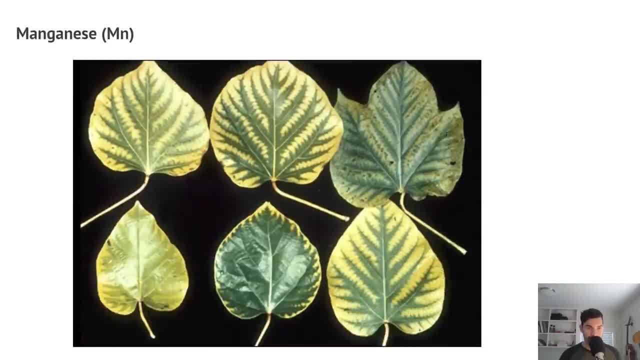 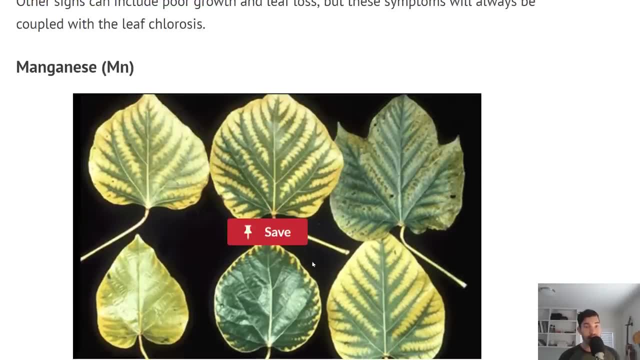 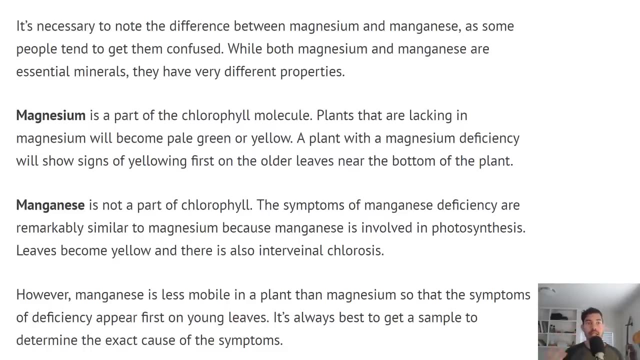 Right, And so that's kind of what you're seeing with leaf chlorosis: manganese- Look at this deficiency symptom: manganese needed for chlorophyll production. That is an intense deficiency symptom right there. So one thing I have to talk about here is there is a difference between magnesium and manganese. 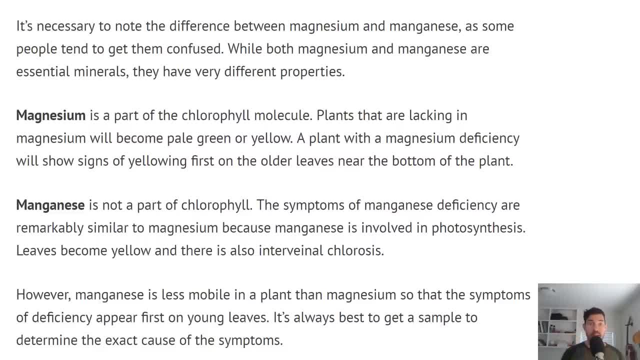 and they're very similar in their sound, but they have a lot of different properties. So magnesium is part of chlorophyll, So plants that are lacking in magnesium will become pale, green or yellow because they are not able to photosynthesize properly. 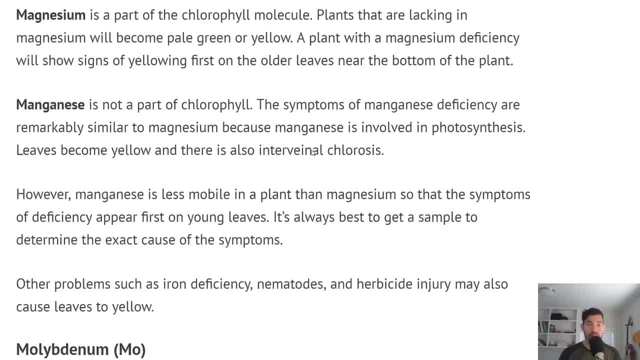 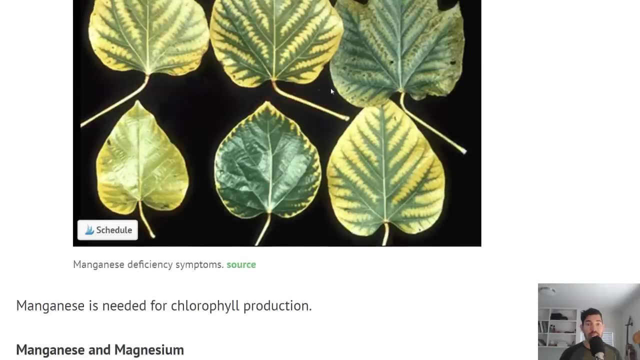 Manganese is not part of chlorophyll, And so when you're seeing a manganese deficiency, what you're going to see is very similar to a deficiency in magnesium, because manganese is involved in photosynthesis and leaves are become yellow, which you see right here. 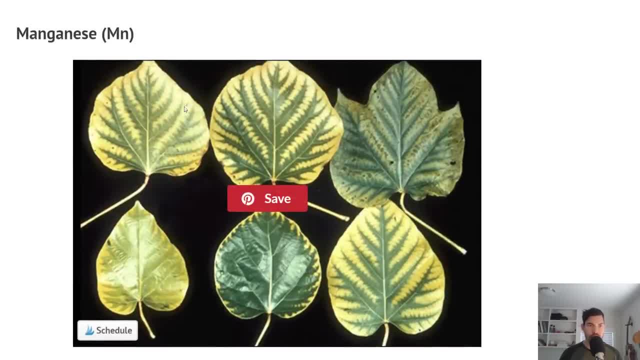 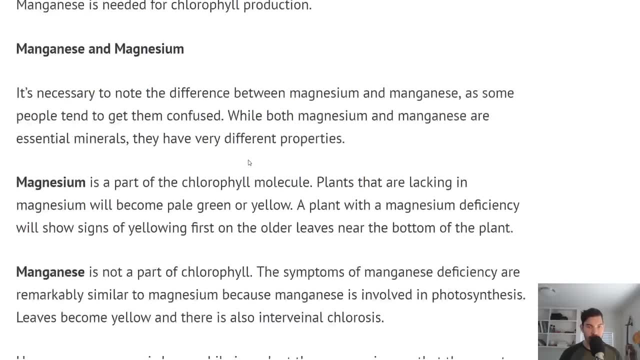 It's very stark, though. This is a very stark difference: Deep pale yellow here, And then you have this green hugging around the veins of the leaves And that's how you can tell you have a manganese deficiency. So manganese is going to be less mobile. 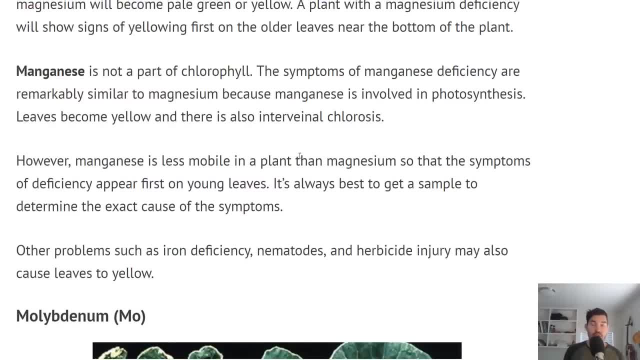 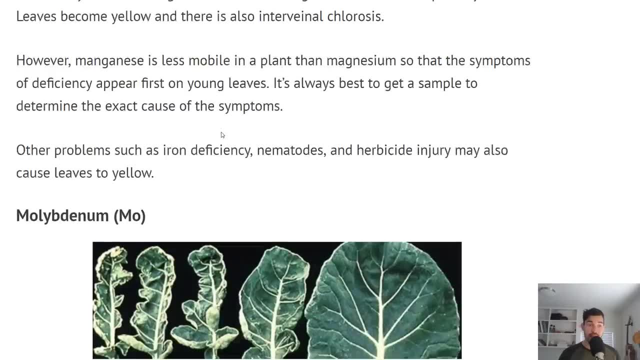 And if we've learned anything in this video, we know that a less mobile nutrient is going to show up on new growth, not old growth. That's how you're going to be able to tell the difference between, maybe, a magnesium and a manganese deficiency. 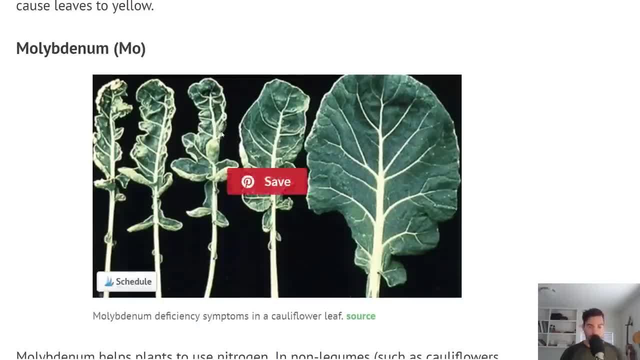 All right, now we have molybdenum. I believe that's what it is Right. That's how you say it. So here is a deficiency symptom: on a cauliflower leaf, You can see this curling and shriveling. 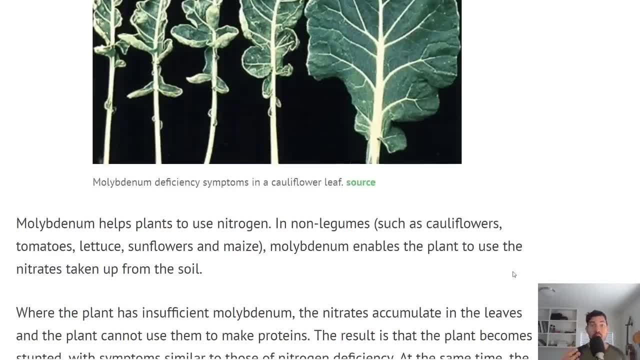 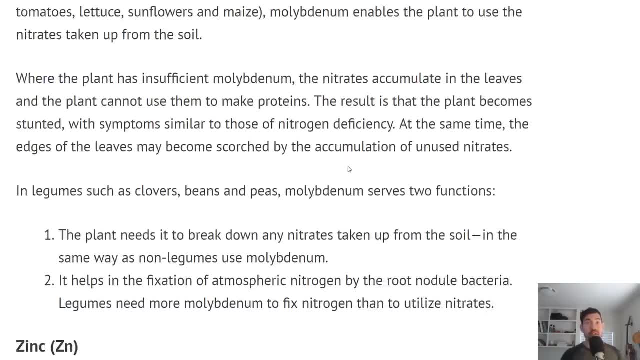 Molybdenum helps plants use nitrogen. So in a non legume like a cauliflower, molybdenum enables the plant to use nitrates taken up from the soil. So if you're going to have insufficient molybdenum in your soil, 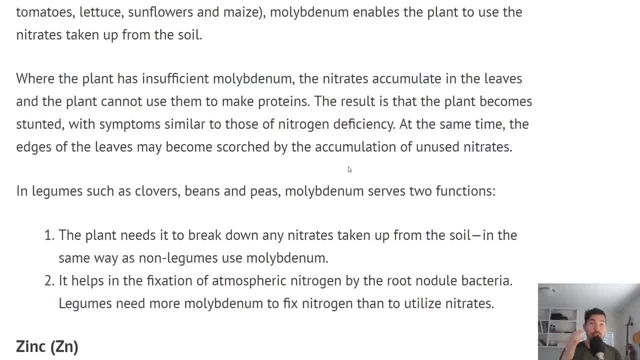 then nitrates are going to accumulate in the leaves because the plant can't use them Right, And so then you have stunted growth, with symptoms very similar to nitrogen deficiency, because the plant molybdenum. the absence of molybdenum is meaning that the plant cannot use the nitrogen. 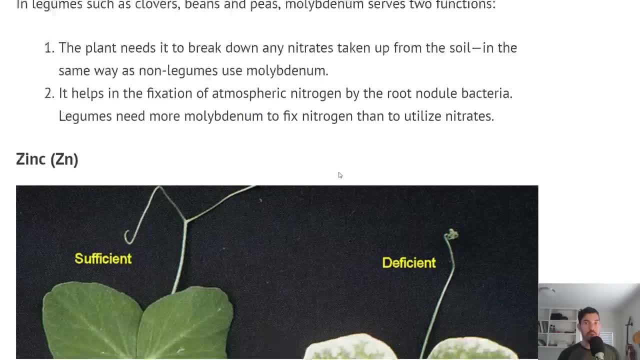 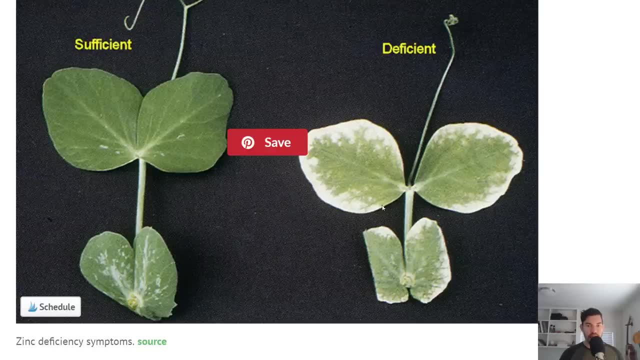 right. So you're going to get a nitrogen deficiency because of that. So let's move on zinc. here is zinc deficiency symptoms, and you're seeing a whitening of the leaves on the outer edges and sort of a modeled appearance right there. That is a symptom of zinc deficiency. 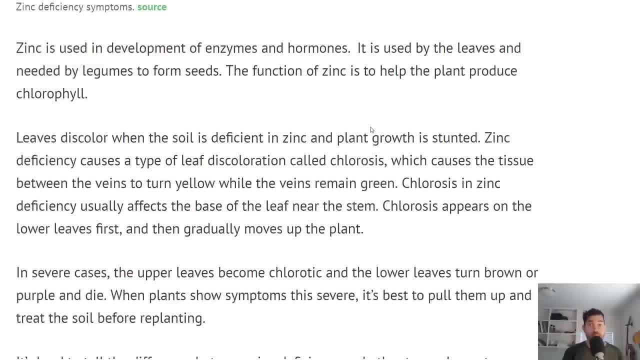 So zinc is used- excuse me- in the development of enzymes and hormones. So it's used by leaves needed by legumes to form seeds. It leaves are going to discolor, The plant growth is going to be stunted. Uh and again. 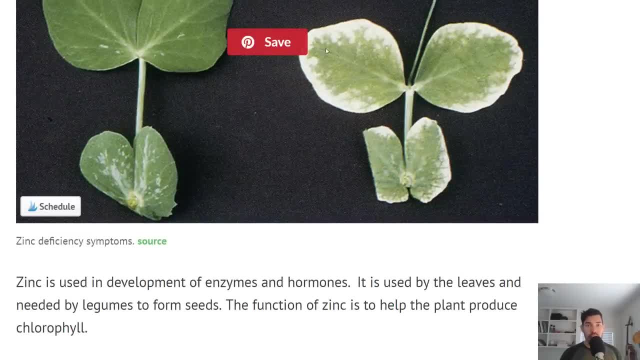 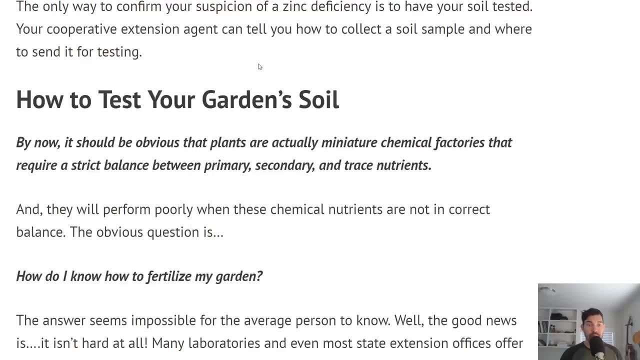 you're going to get chlorosis, So the veins will remain green and the tissue, the leaf tissue itself is going to become whiter. All right, there we go. Those are the nutrients that a plant needs. a brief rundown of what they do in the plant. 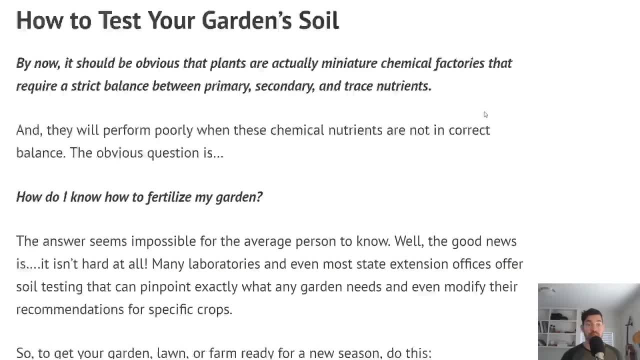 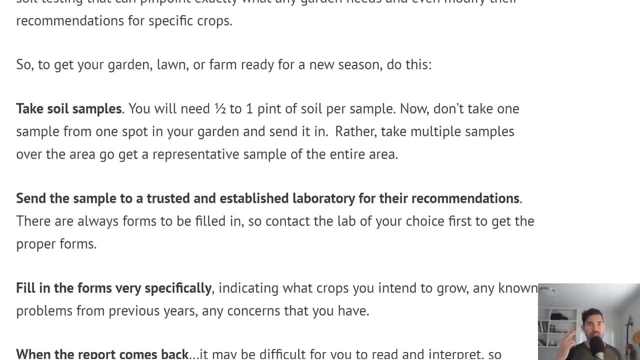 And then, if they're missing, what's going to happen to the plant as a result? Now, there's a lot more information about soil testing and things like that. you can check out epic gardeningcom for that- But I wanted to do this video and I know I've done a lot of these lecture style videos lately. 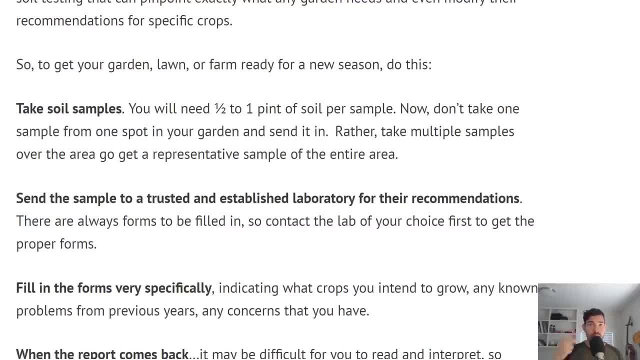 Um, but we're going to get back to live action soon. I've got some mushroom stuff, some micro green stuff, some hydroponic stuff, some soil test stuff coming up, but I wanted to get this one out there cause I think it's important and I really hope it's valuable.